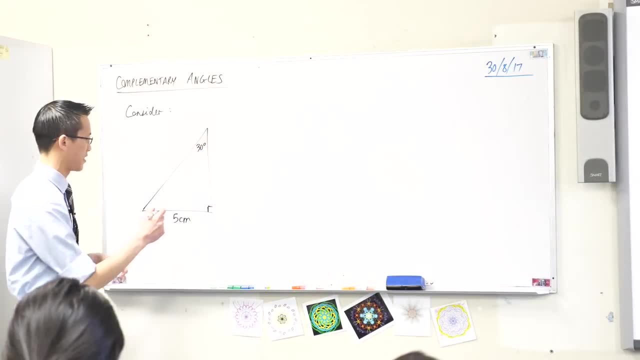 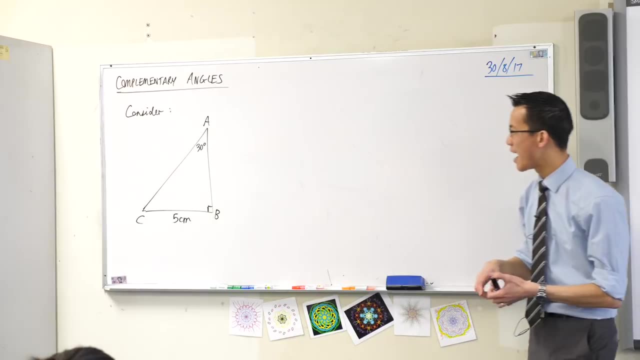 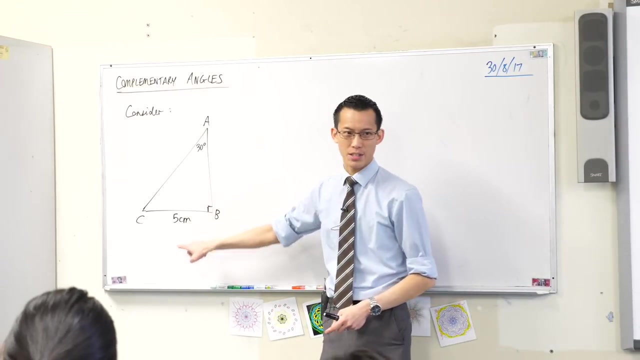 I've got a triangle here for us. Let's label some sides and angles, shall we? Let's call this A, B and C. So in triangle ABC we have a right angle in the corner. that's what we've been so far working with within trigonometry. We also have an angle and a side. 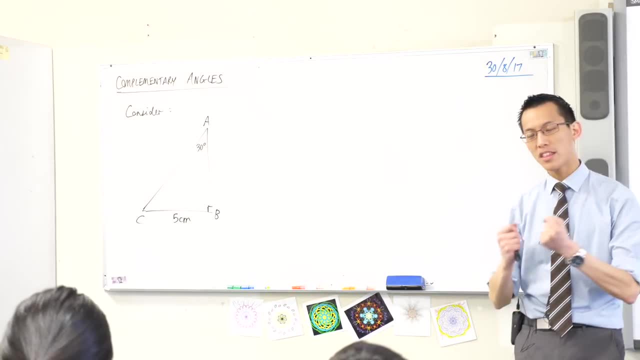 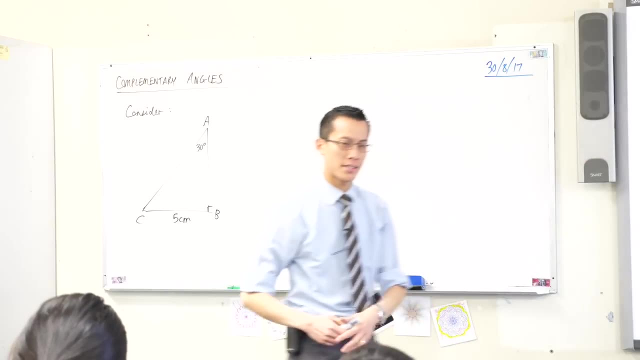 Now, on the basis of this information, with trigonometry in our pocket, we can actually work out absolutely everything about this triangle You know. in Pythagoras, if you wanted to know, say, a third side, you had to know two of the other ones. 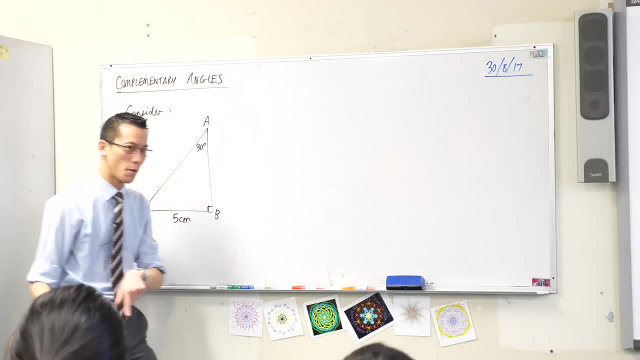 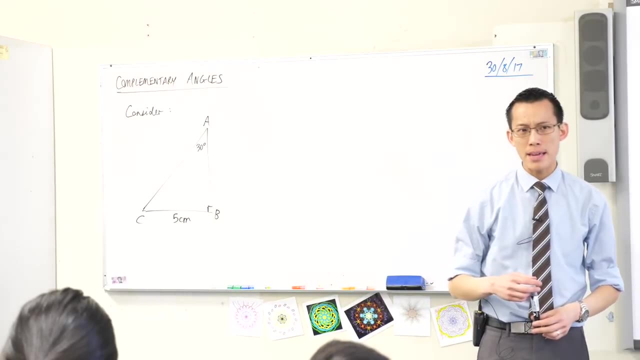 or if you wanted to know this one, you had to know these two. but with trigonometry you don't need that much information, this is enough. For instance, can you help me work out what A B is? What kind of equation would I write to help me work out A B? 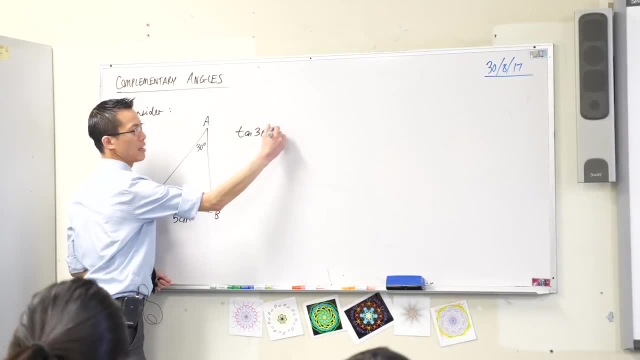 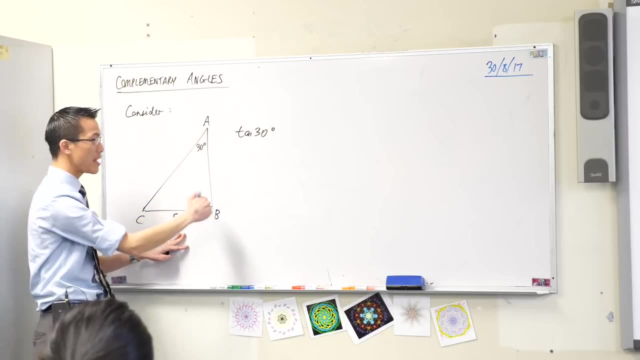 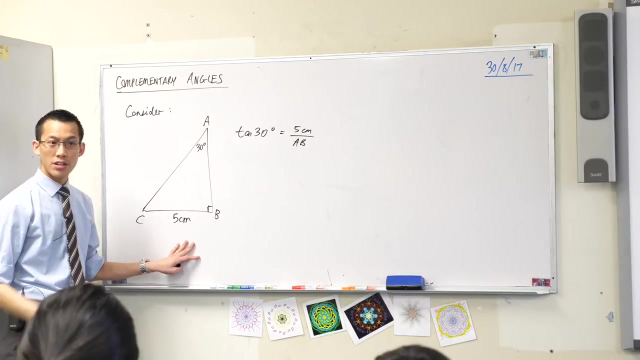 tan 30. Let's write that down. Tan, of course, is opposite on adjacent, so that's this guy over this guy. So tan 30 is 5 centimetres over A B. So you can see, I can rearrange this a teeny bit, in fact. 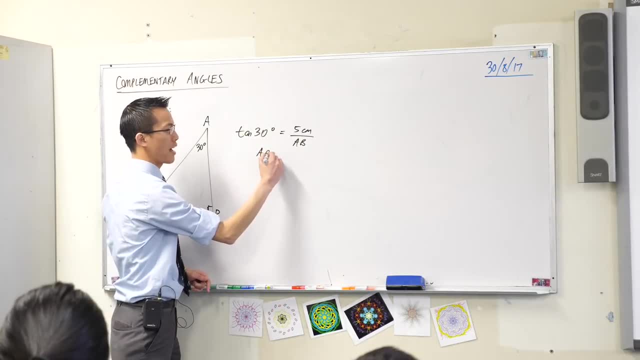 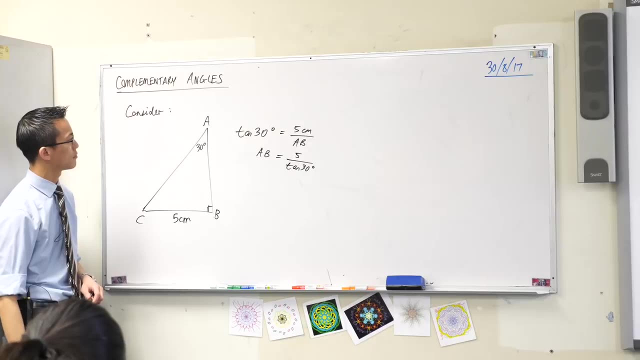 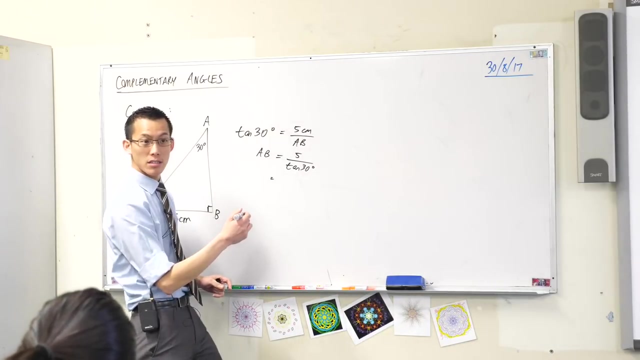 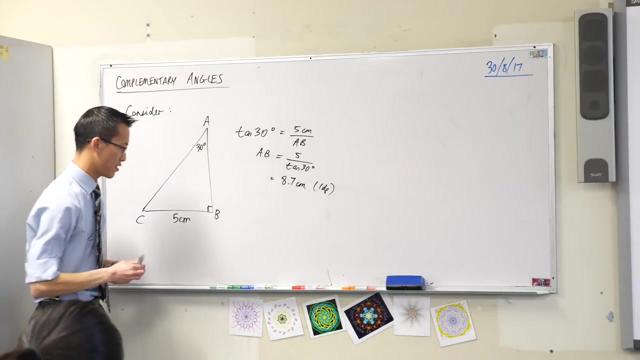 these guys are going to end up swapping places. With your calculator you could find this like: so: Can you tell me what that is? Can you give me, say, one decimal place that'll do 8.7? So with that information I can put this guy on here- 8.7.. 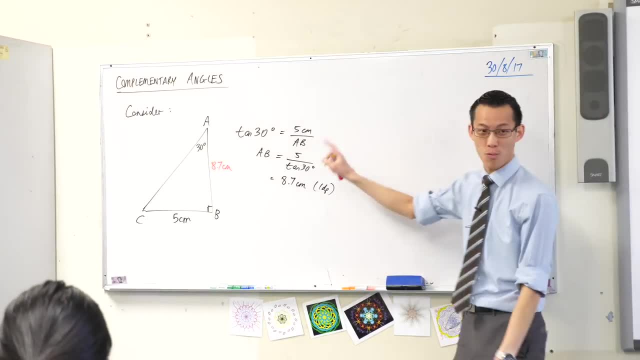 Now I could use Pythagoras. that's what we're so used to doing when you see a right angle triangle and you've got two sides. but I'm going to try and keep on using trigonometry because it seems to work pretty effectively. So I'm going to try and keep on using trigonometry because it seems to work pretty effectively. 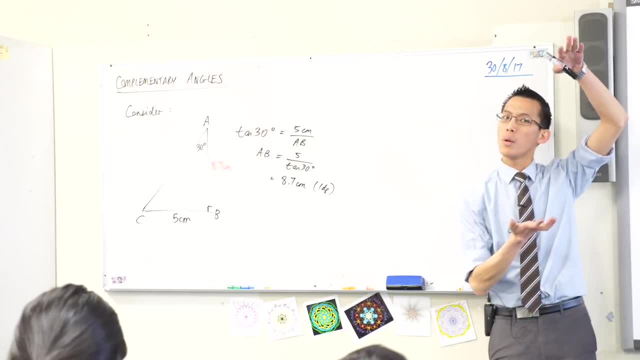 So I'm going to try and put this right. it seems to work perfectly here. If I didn't want to go to A B, what would I write? what new equation could I write to help me get A C? oh Aaron, what do you say? 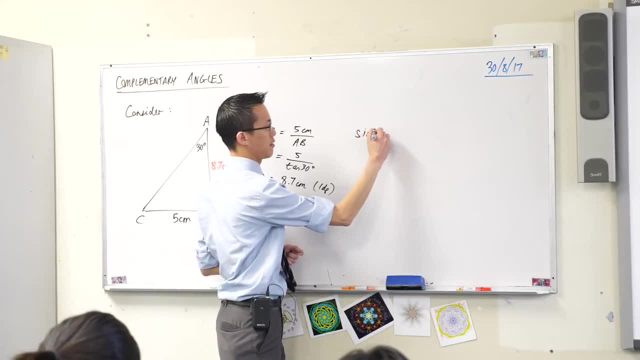 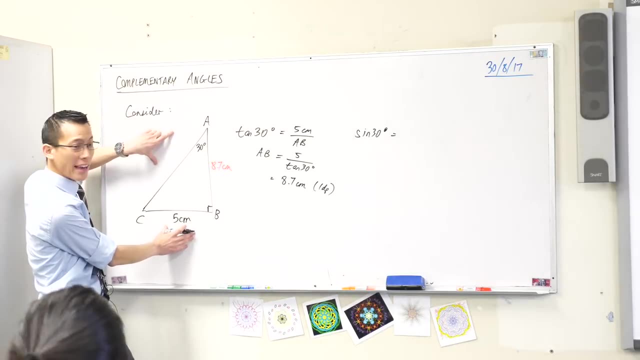 For a sine 30. Sine 30?? Let's all write that down. Sine, of course, is which pair of sides All Hyung- vé. Sine, of course, is which pair of sides Off opposite, Off opposite, Off opposite. on hypotony, So I can write 5 on A, C. 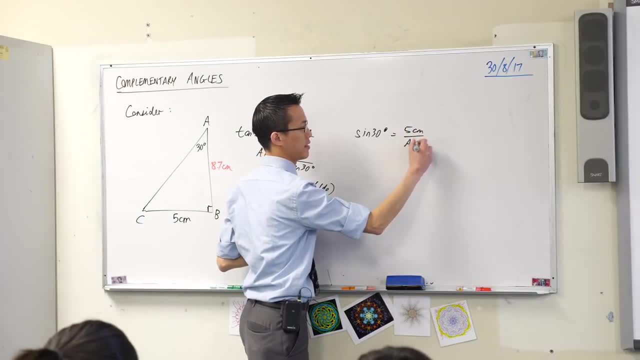 On a C, Just like before. I can rearrange it to the five on the lowest and minus five On a C. As I quite said, I can write 5 on the A C. so what does that tell me? 5- value of aspirations. 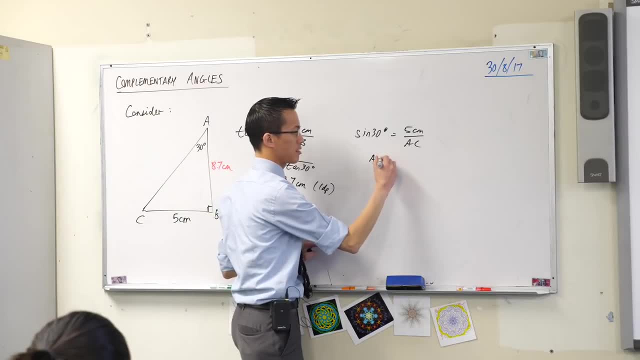 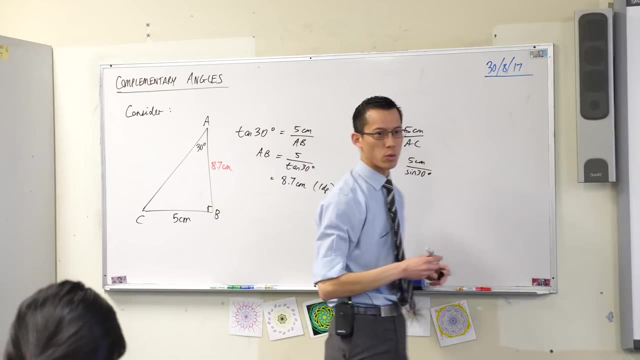 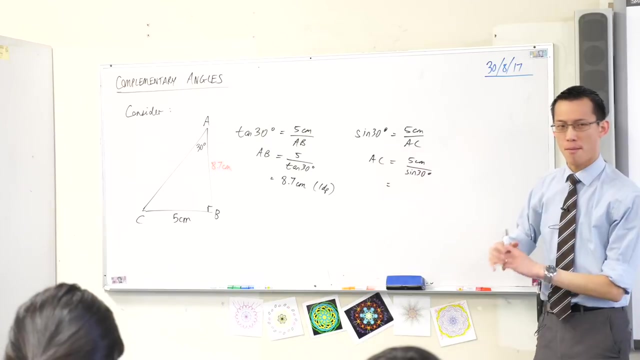 5. value of vierages. 5. value of Collection. I can rearrange a teeny bit to get this and, interestingly, when you press equals- unlike normally when you get strange, unusual decimal rubbish happening- when you get this, if my memory is right, you should get exactly 10. huh, that's. 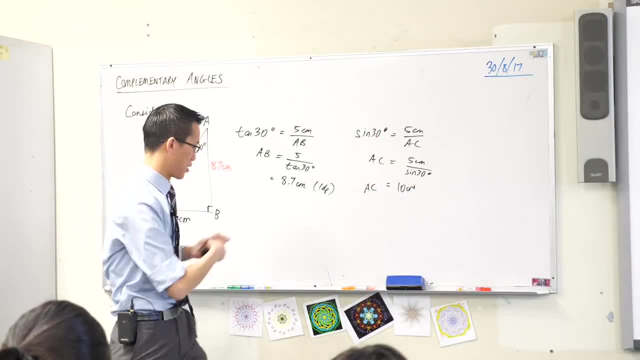 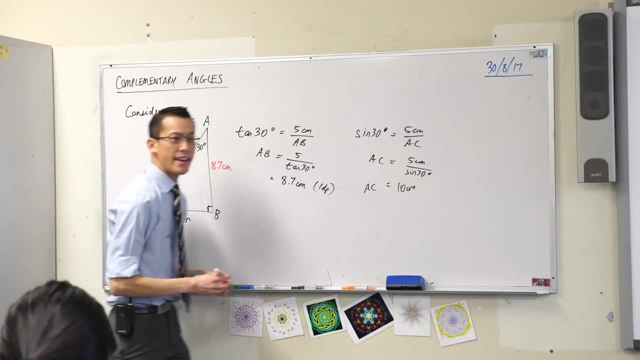 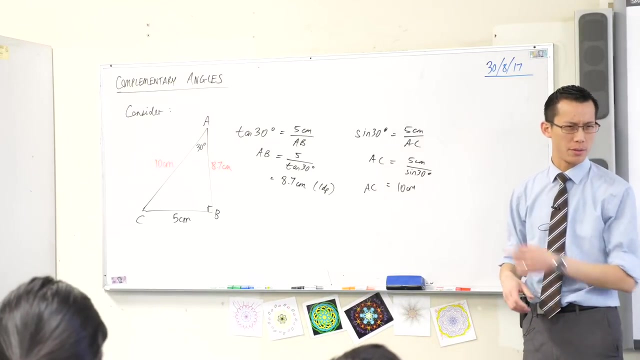 interesting. so we've got this number and we can put it onto our diagram. now I've got three sides in a triangle and I know all of them, and they're also three angles in a triangle. I almost know all from this. one of those is missing, which. 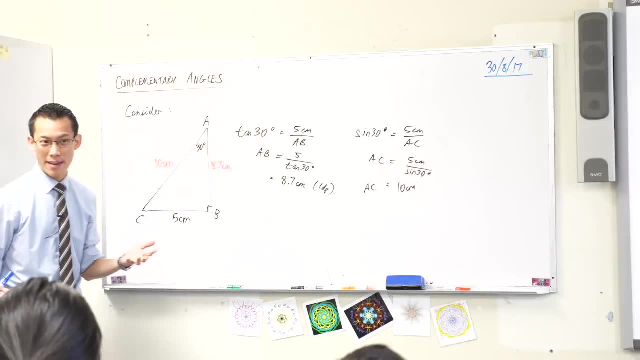 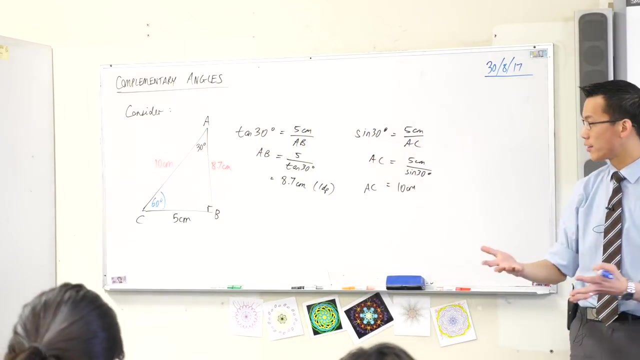 one. ah yeah, ACB, ACB or BC a have a look at the angles that we've got. what is the size of this angle? it's gonna be 60 degrees. how did you find that? angles in a triangle? the angle some of the triangles 180 degrees. 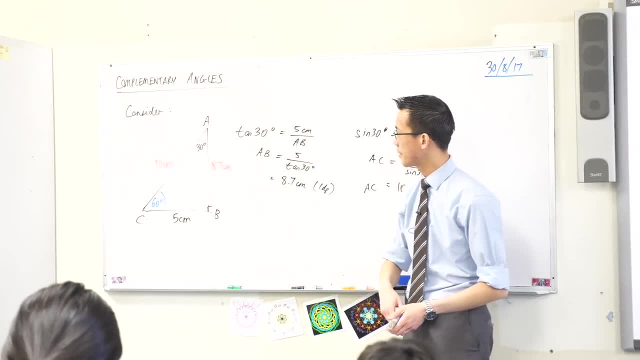 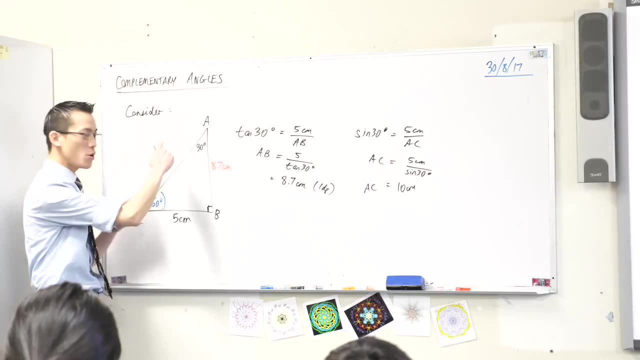 so ž. So 30 plus 60 plus 90,. okay, Now you might also notice I gave you this title right Complementary. That wasn't by coincidence. Hardly ever is The two angles here that are interesting in this triangle. 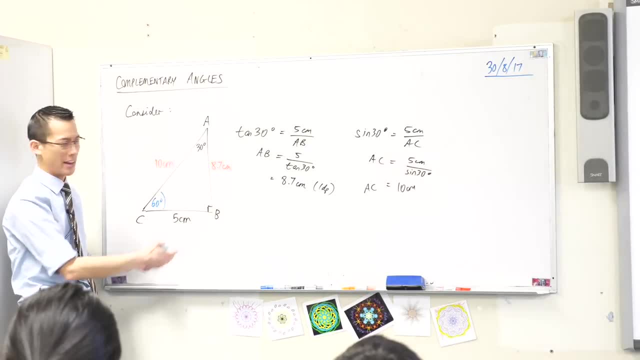 that can change, because we've been dealing with right-angled triangles, So it seems to be always a right angle there. These guys are complements of one another. They add up to 90 degrees. Do you see that They have to, because there's 90 already here? 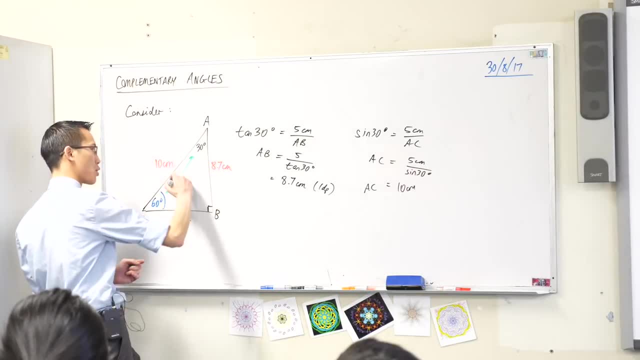 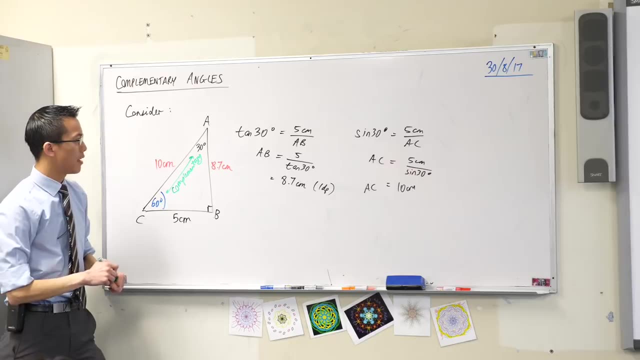 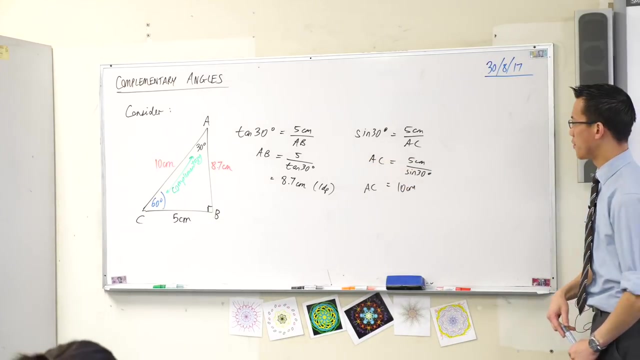 There's only 90 degrees left in the triangle to make up all the rest, So I'm going to write here complementary. Okay, Now we have tan 30,, we have sine 30. And now we know there's a 60-degree angle over there. 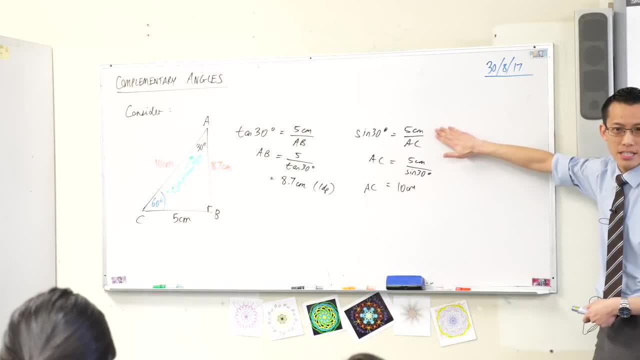 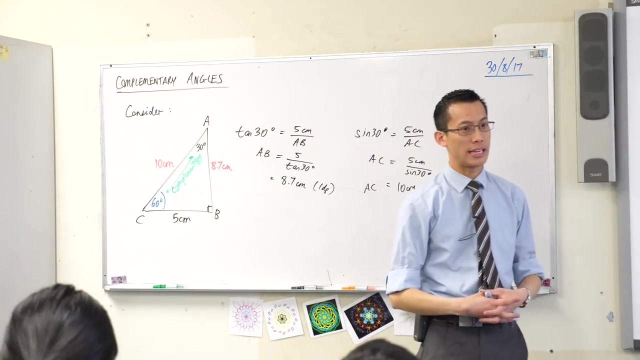 But what I want you to notice is see this: 5 centimeters on AC. We came up with that as opposite on hypotenuse, Opposite on hypotenuse, But I can also think of it as adjacent. So I can think of it as adjacent on hypotenuse if I change the angle I'm looking at. 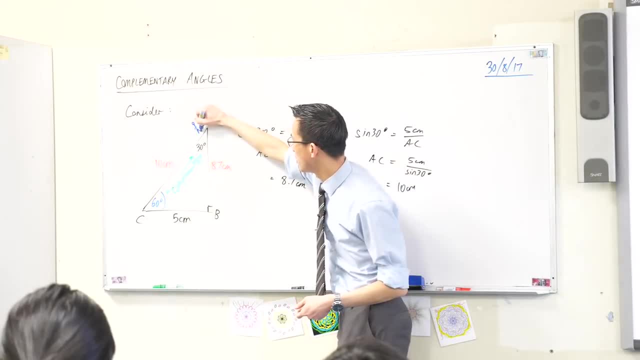 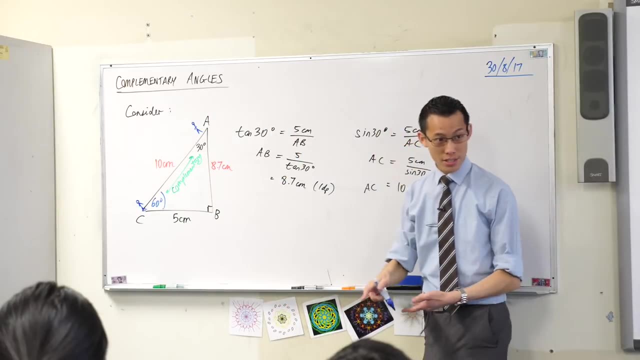 Right, Remember I told you trigonometry is about position. So if you change your position from standing up here, that's where the 30 degrees is. Now I want to stand down here. Do you see now if I'm from the perspective of angle ACB? 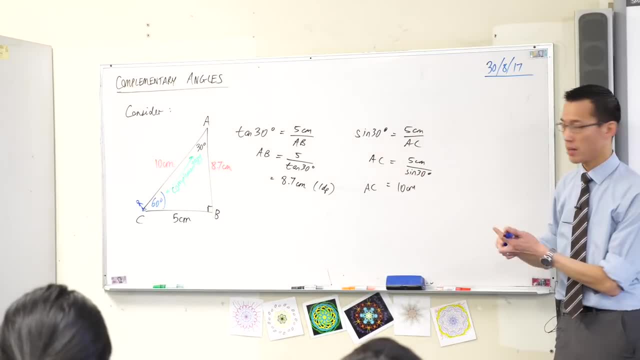 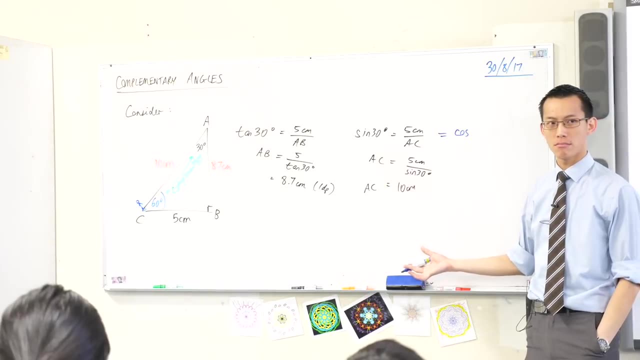 This is not opposite on hypotenuse, It's adjacent on hypotenuse, Do you agree? So which ratio is that? That's cos, That's cos. I'm standing at a new angle. And what is its size? It's 60.. 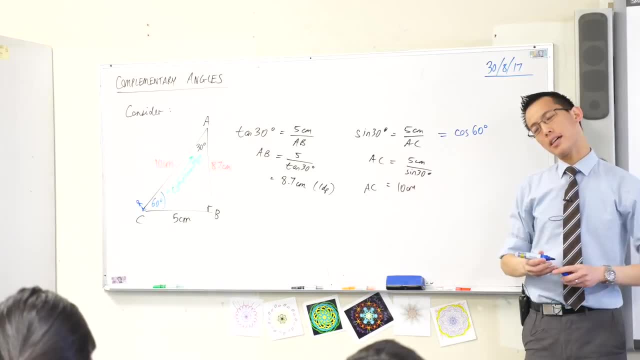 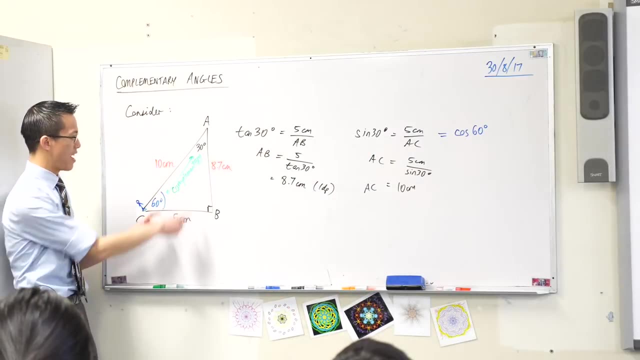 It's 60. OK, Now it doesn't take that much imagination to realize I could change this triangle. I could like take A and I could squash it down a little bit, And all these angles and sides would all change accordingly, right? 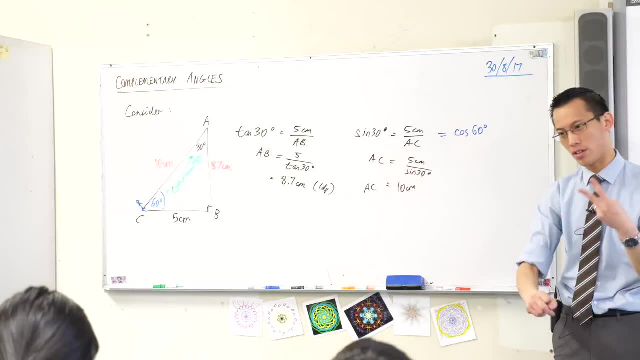 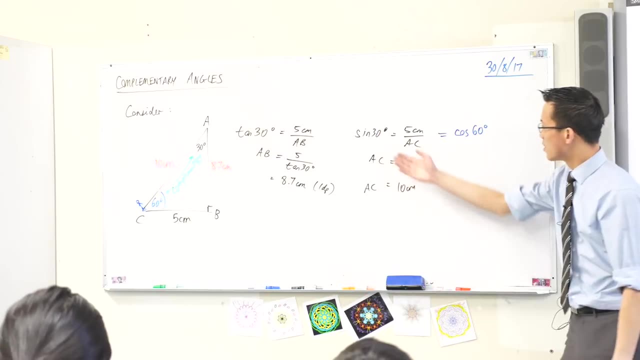 But everything we said about position opposite on hypotenuse, adjacent on hypotenuse, they'd all stay the same. I haven't changed its rearrangement, I just made it smaller or bigger. So all of this would be the same, just with slightly different angles. 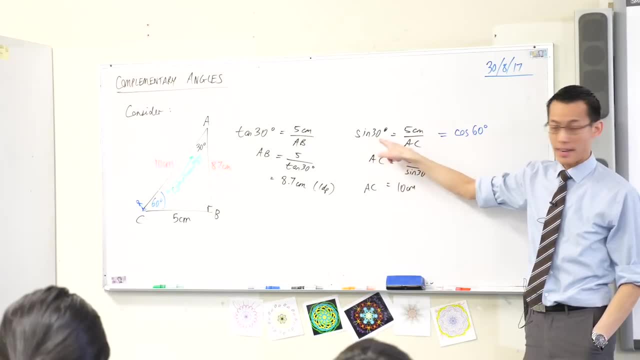 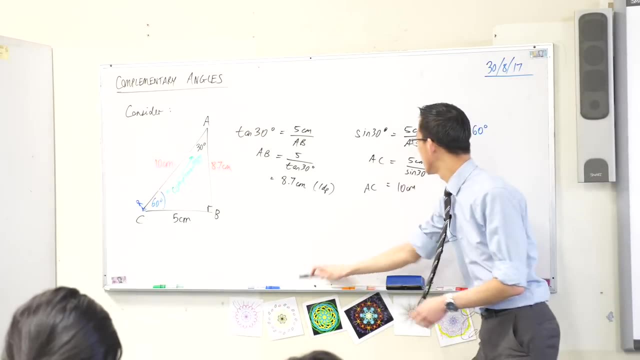 Just different numbers. OK, So here go to your calculator. now See how you say: sine 30 equals cos 60, right, Your calculator can verify this for you. Both of them should give you a half. Is that what you find? 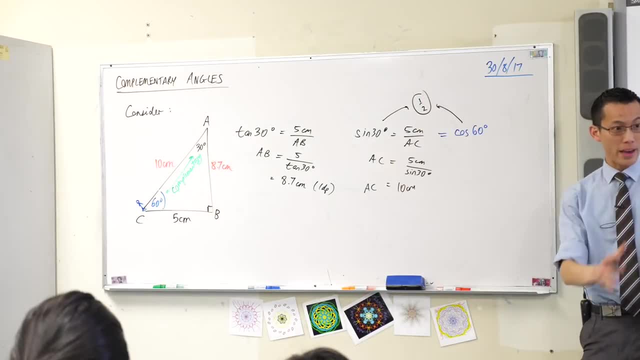 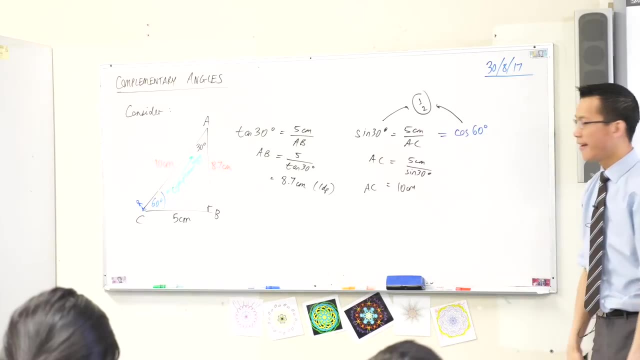 Yeah, A half, A half, Which, by the way, is the reason why this came out to be see 5 over 10? It's exactly a half, Not just close to it, exactly Now, if I squash this triangle down, if I made it like shorter, OK, this 60 degree angle. 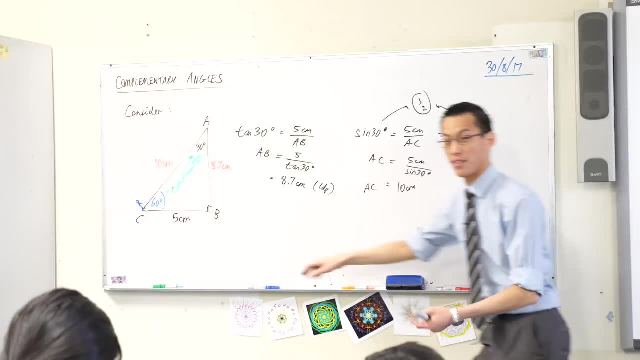 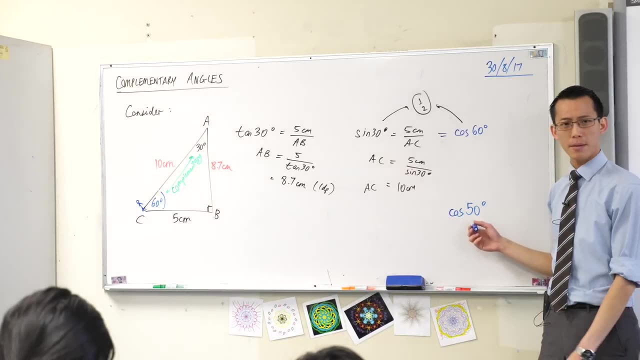 might be something smaller. Suppose it ended up being instead of 60, suppose it might be 50.. If this angle became smaller, what would happen to the other angle Side- sorry angle BAC. What would it become Bigger? 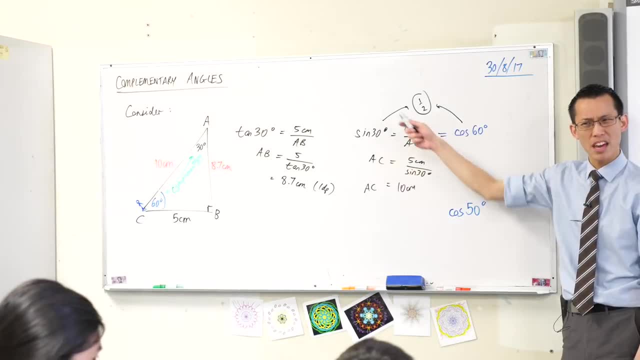 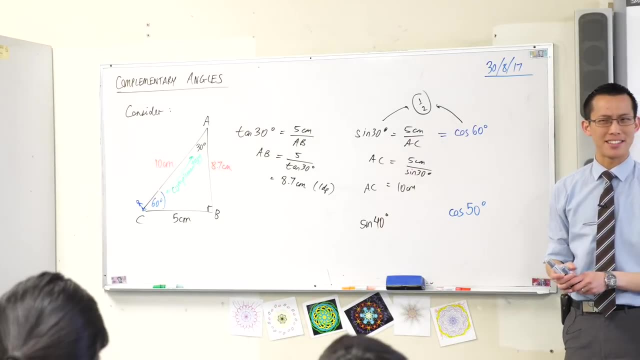 It would not be. yeah, it would be bigger than what it was before. It wouldn't be sine 30,, it would be sine 40. Now, 40 and 50 don't give you nicely numbers, but with your calculator and I'd love it. 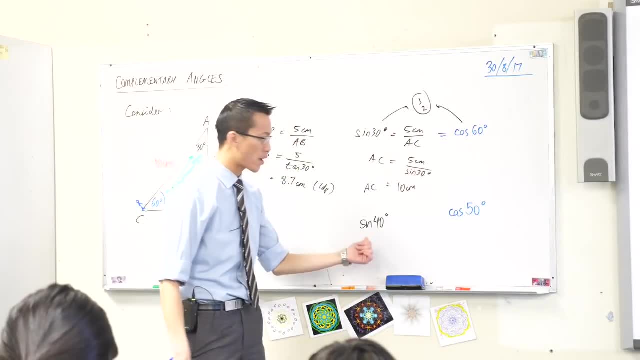 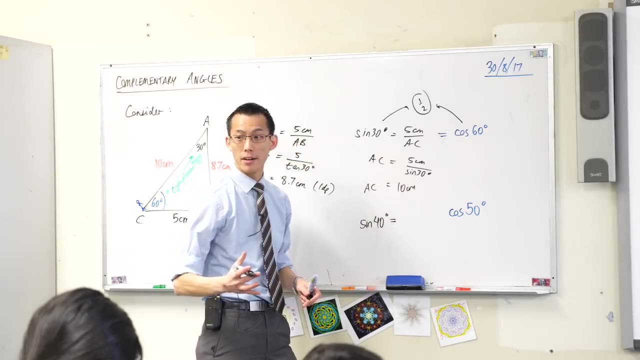 if the two people like if you're paired up, I'd love one of you work out sine 40, and the other one will work out cos 50.. What do you get? What's the number That'll do? 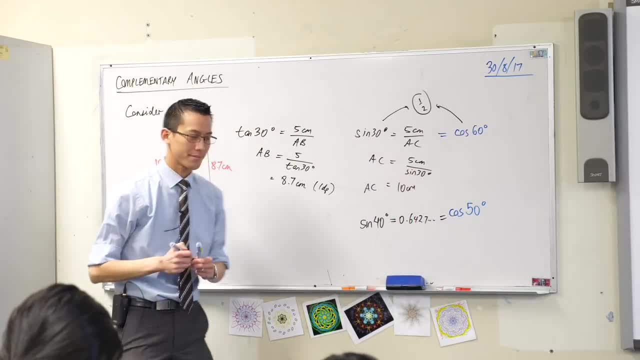 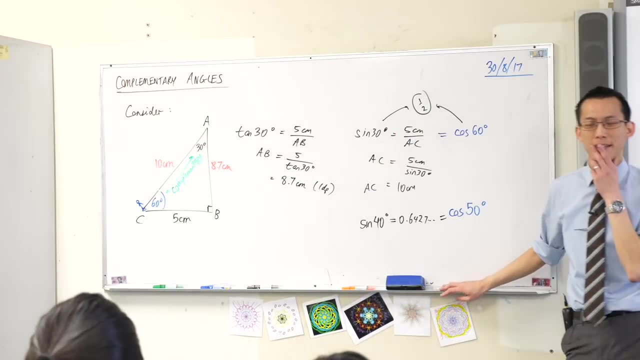 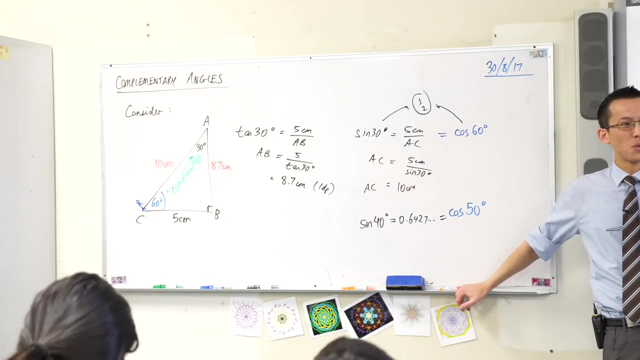 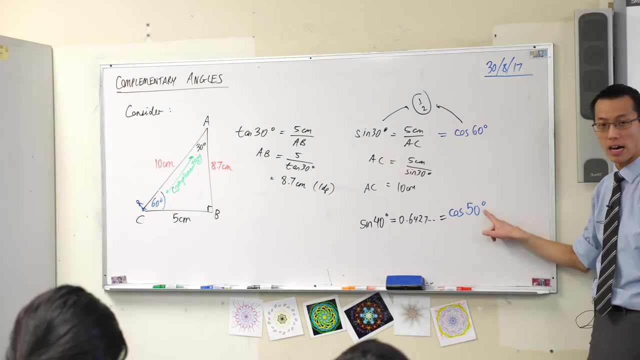 That's fine, OK. So, shh, Stay with me a tenth. So what you're noticing is, if I squashed this triangle or stretched it out, I could make this angle rather than smaller, I could make it bigger. 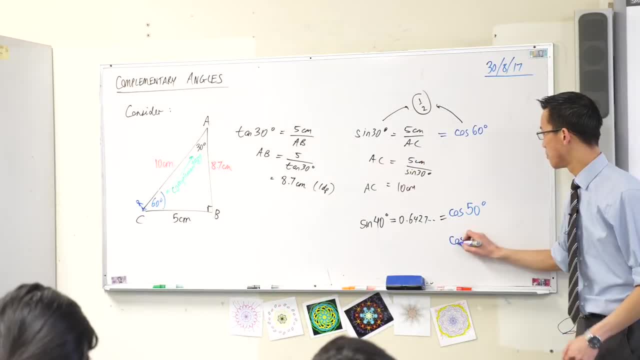 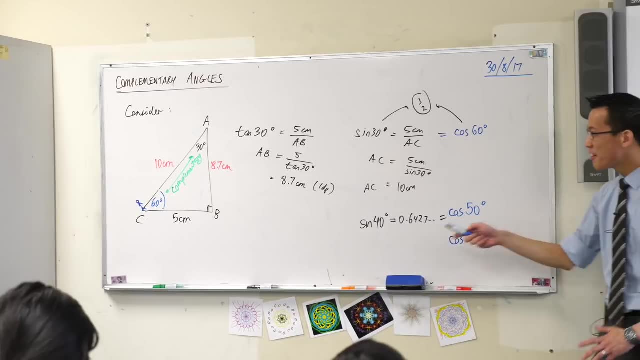 Give me another angle that could fit inside this triangle, Bigger than 60.. Anything you like: 70.. 70. You guys are so original. OK, If this is 70, then the other angle is always going to be complementary, so it'll be 20.. 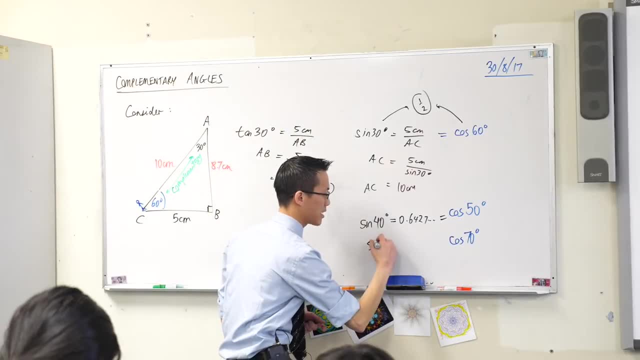 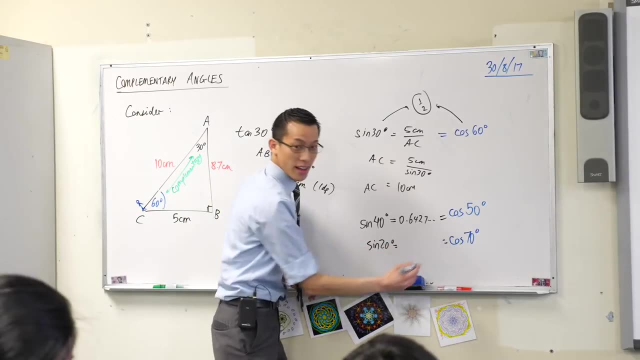 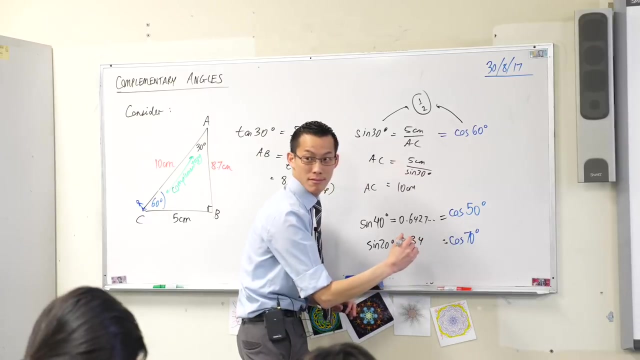 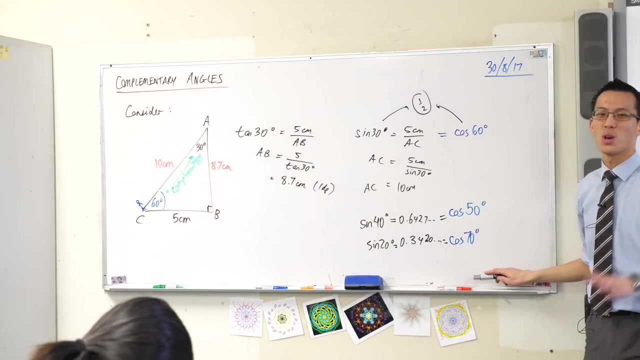 Right. Well, again, go ahead, try it with the person next to you. Test out sine 20 and cos 70. And you should find that both of them are Zero point Two, zero, OK. So what's going on here? 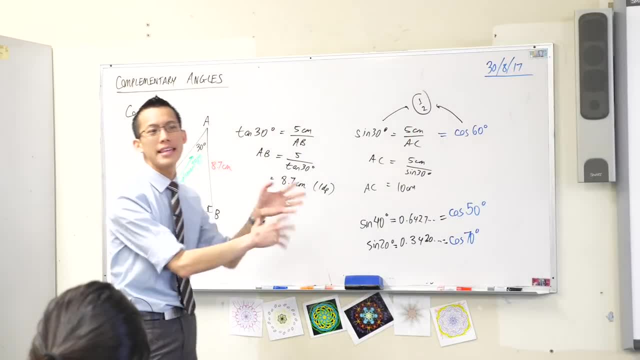 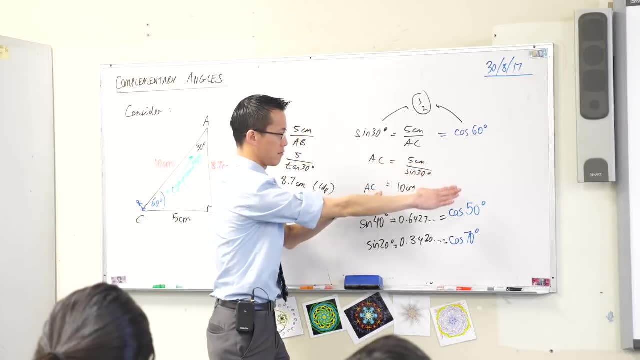 You guys know- I have an obsession with names, right- Why things are called what they are. OK, What you're noticing is that if you have complementary angles- angles here 30 and 60,, 40,, 50,, 20,, 70,, 5 and 85, so long as they're complementary- 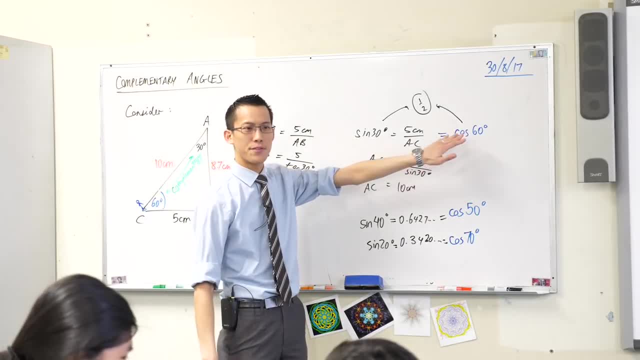 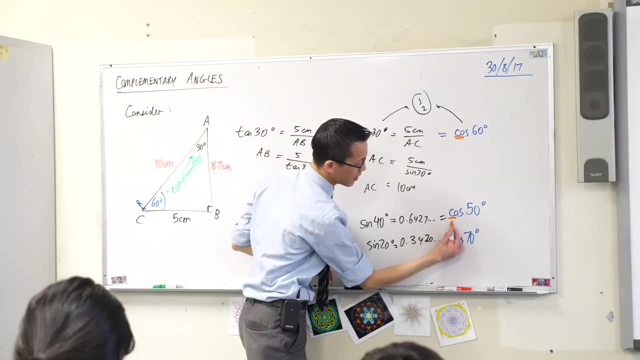 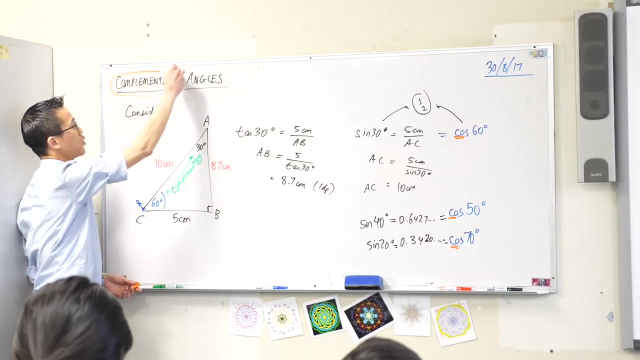 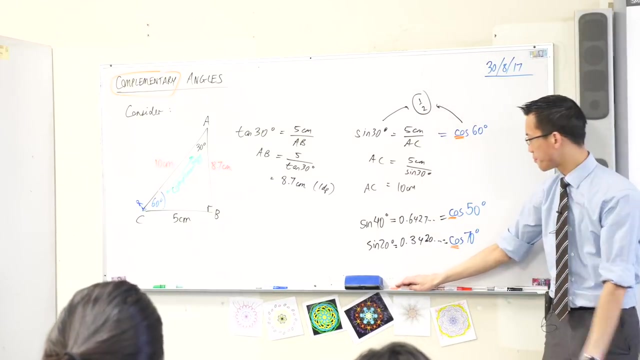 you find the sine of one is the same as the cosine of the other And in fact that's exactly what cosine stands for. The co is short for complementary. OK, Yes, So when we say the cos of some angle right, what we mean is it's the complement of sine.